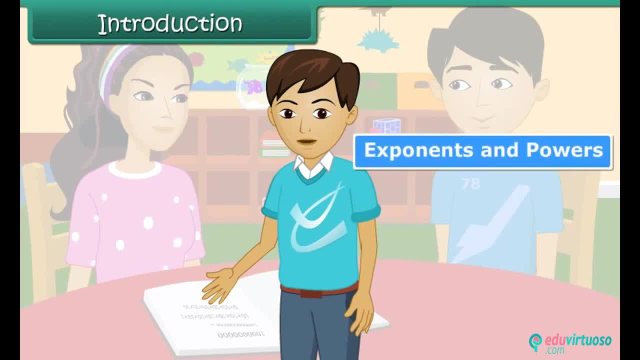 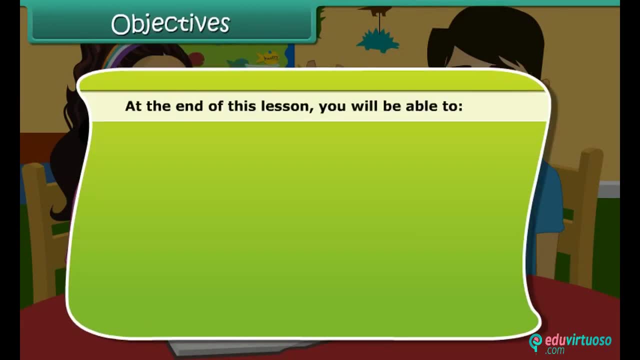 In this lesson, you will learn about exponents and powers Objectives. At the end of this lesson, you will be able to Express a number in exponential form, Identify the base and exponent of a number expressed in exponential form, Compare numbers expressed in exponential form. 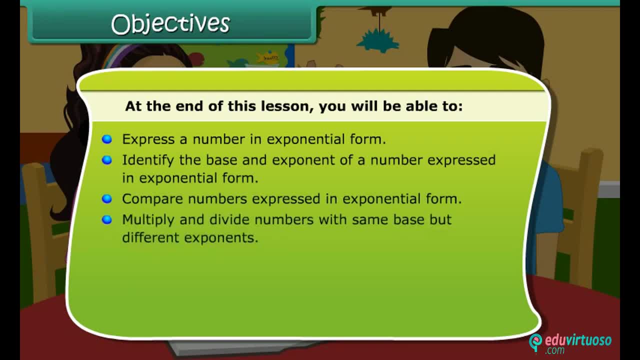 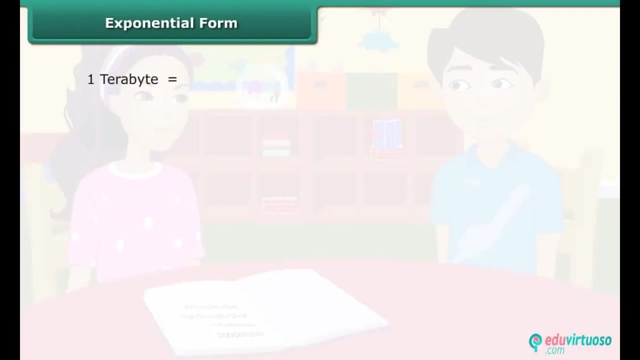 Multiply and divide numbers with the same base but different exponents. Multiply and divide numbers with the same exponent but different bases. Raise an exponential number to a power. Raise a number to the power: 0 Exponential form. You heard Dhruv tell Varisha that 1 terabyte is equal to. 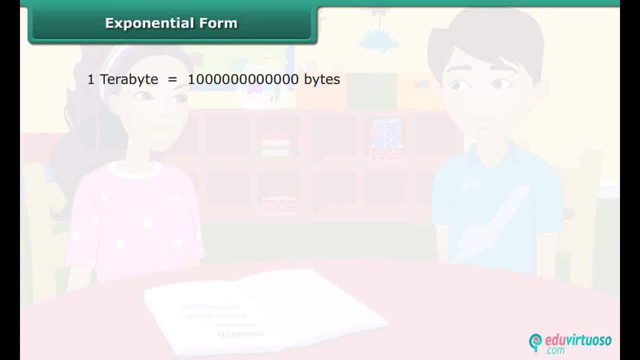 When expressed so, the number on the right is difficult to identify and use. Hence such large numbers are expressed in exponential form to reduce their size and make comprehension easy. 1,0,0,0,0,0,0,0,0,0,0,0,0,0,0,0 is nothing but 10 multiplied 12 times. 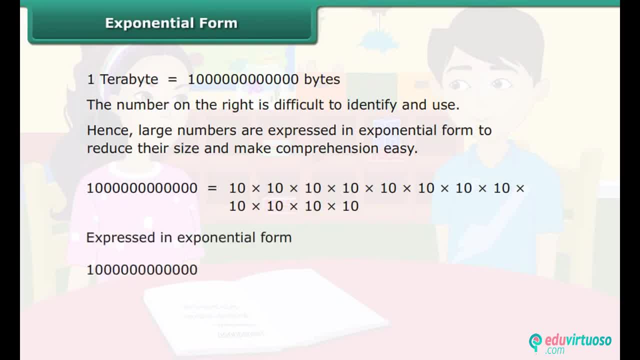 We use this knowledge and express 1,0,0,0,0,0,0,0,0,0,0,0,0,0,0,0,0,0 in exponential form, as an exponential formula to interpret the expression. 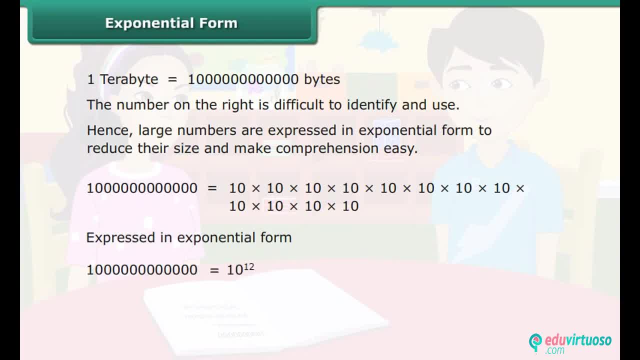 exponential form as 10 raised to the power 12.. Therefore, as rightly pointed out by Dhruv, 1 terabyte may be expressed as equivalent to 10 raised to the power 12 bytes. 10 raised to the power 12 is made up of two. 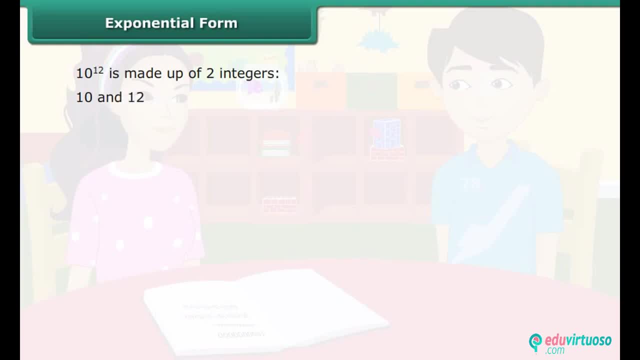 integers 10 and 12.. 10 is known as the base and 12 is called the exponent. We can express large numbers in exponential form by varying the base and the exponent. Look at this number expressed in exponential form: Base is 4 and exponent is 2.. 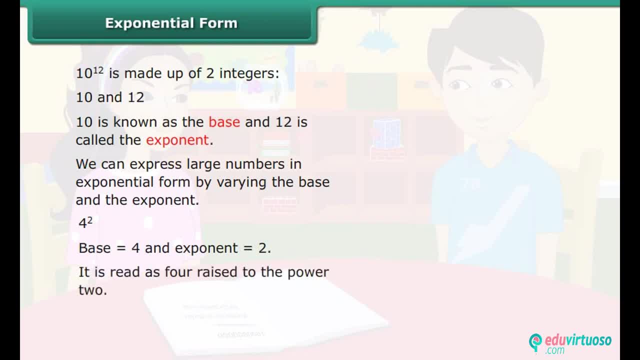 It is read as 4 raised to the power 2.. 4 raised to the power 2 is nothing but 4 into 4.. Hence it is also read as 4 squared. Look at one more exponential number: Base is 4 and exponent is 3.. 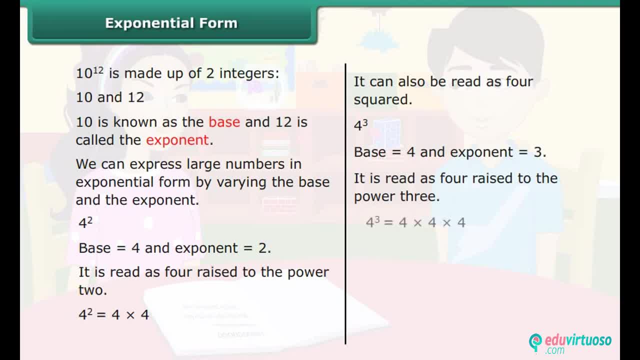 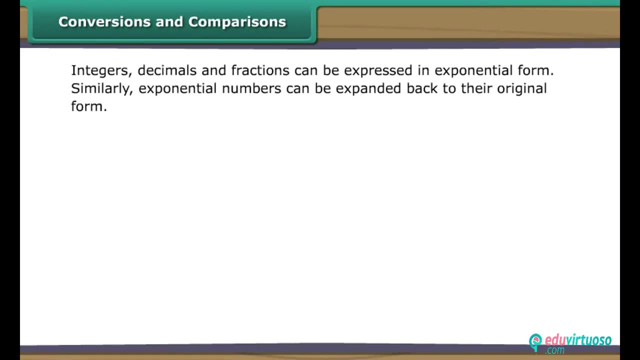 It is read as 4 raised to the power 3.. 4 raised to the power 3 is nothing but 4 into 4 into 4.. Therefore, it is also read as: 4 cubed. Conversions and Comparisons, Integers, decimals and fractions can be. 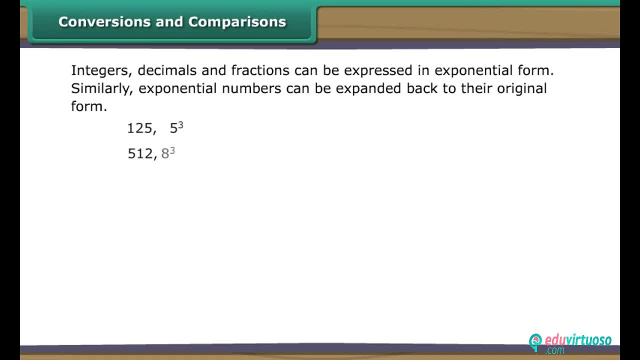 expressed in exponential form. Similarly, exponential numbers can be expanded back to their original form. Exponential numbers can also be compared in much the same way as integers, fractions and decimals are compared. Let us take a look at Conversions and Comparisons of exponential numbers, one by one. 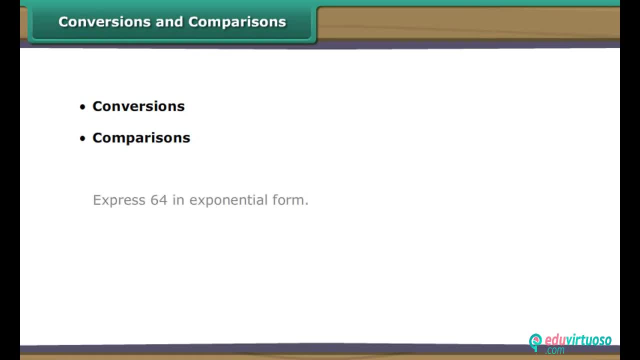 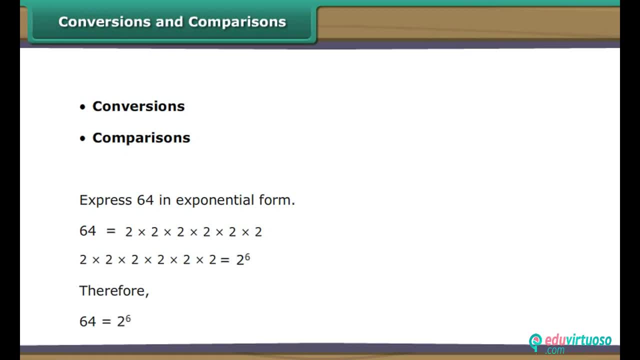 Therefore, 64 is equal to 2 raised to the power 6.. Let us now expand 37456 and express it in exponential form. 37456 can be expanded as 30,000 plus 7,000 plus 400 plus 50. 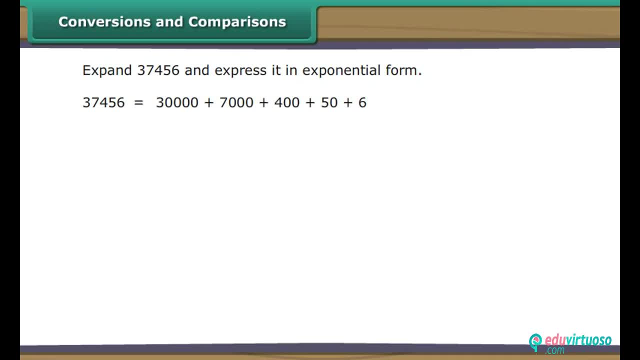 plus 6.. Which is the same as 3 into 10,000, plus 7 into 1000, plus 4 into 100, plus 5 into 10 plus 6.. Which can also be written as 3 into 10 raised to the power, 4 plus 7 into 10. 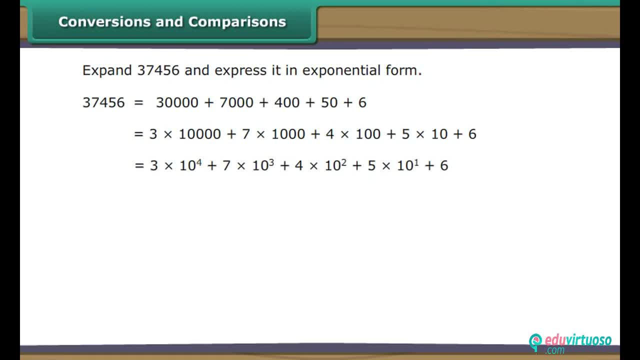 raised to the power 3 plus 4 into 10. raised to the power 2 plus 5, into 10 plus 6.. Let us try and express 196 in exponential form. Let us first express it as a product of its prime factors. 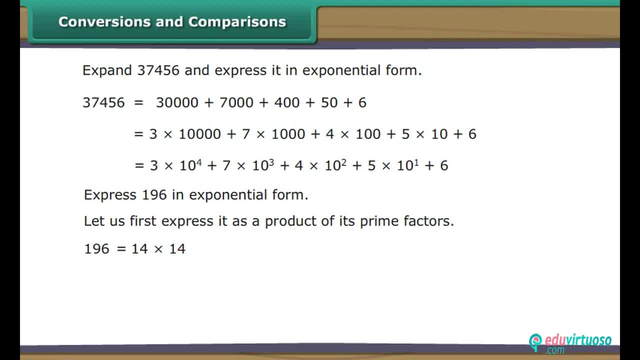 196 is equal to 14 into 14, which is the same as 2 into 7 into 2 into 7.. We can rewrite it as 2 into 2 into 7, into 7.. We can now express the prime factors in. 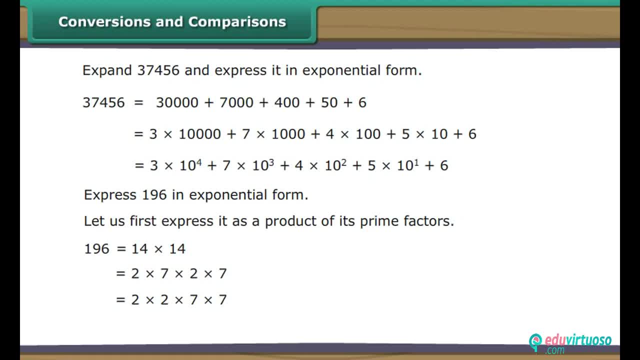 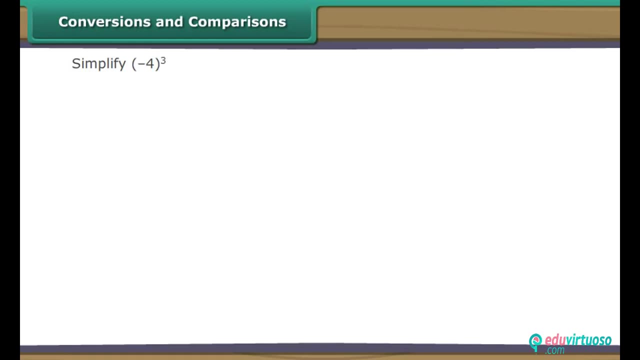 exponential form. Therefore, 196 is equal to 2 square into 7 square. Let us now convert some exponential numbers into their original form through simplification. Let us try to simplify Minus 4 raised to the power 3.. Minus 4 raised to the power 3 may be: 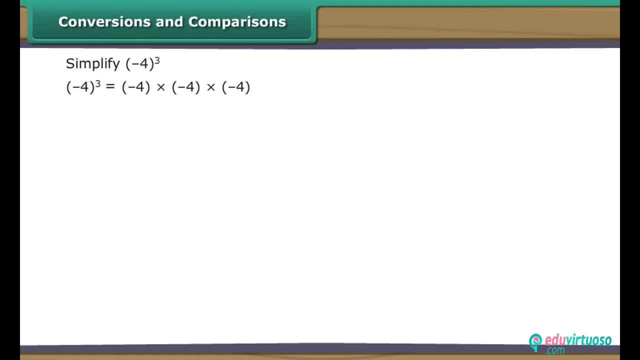 expanded as minus 4 into minus 4, into minus 4.. Which is equal to minus 64.. Simplification of a negative number raised to an odd power gives a negative product. Let us now simplify Minus 6 raised to the power 4.. 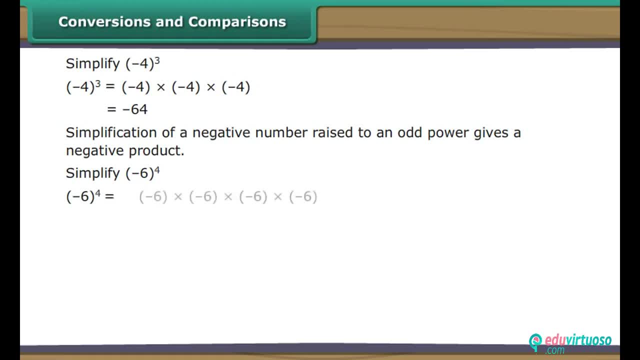 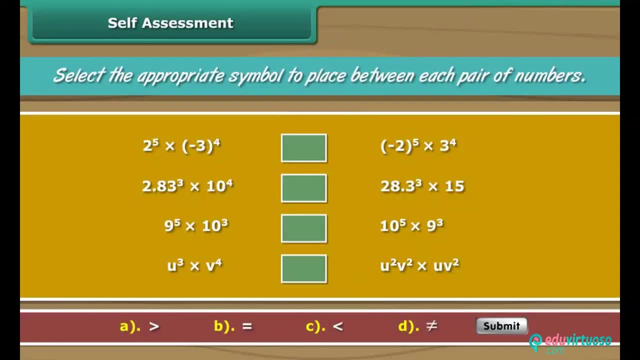 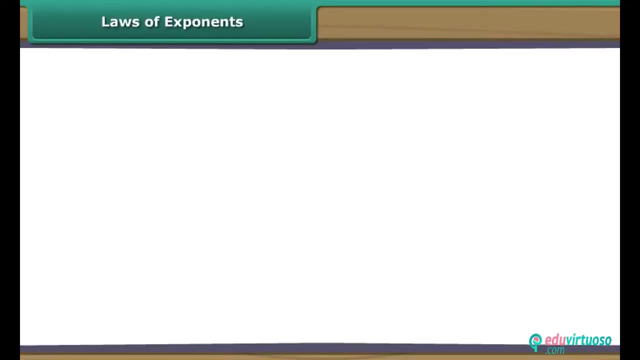 Minus 6 raised to the power 4 is equal to minus 6. assessment: Drag and drop the options in the appropriate boxes. Self-assessment: Select the appropriate symbol to place between each pair of numbers. We can now see that we can now. 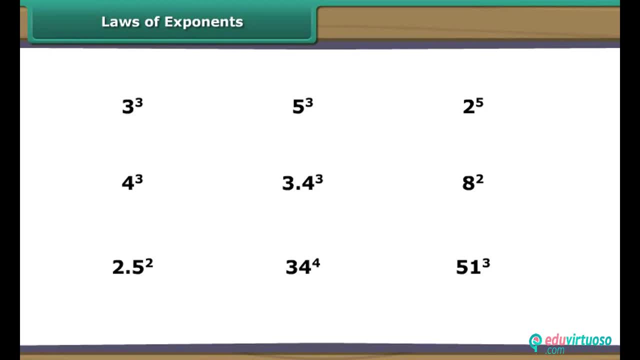 try it. We can now see that we can take the key somewhere else. We can now move on. We can now connect the key to 75, which is the key to 85. But remember, if you connect all the keys in the same number, 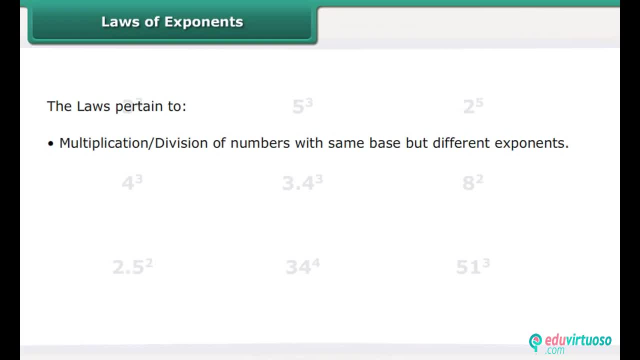 those keys will not be used in the same number. They will be used in the same number. Suppose we take the key to 75. This will now result in a minus 4 raised to the power 4.. Let us turn our attention to the 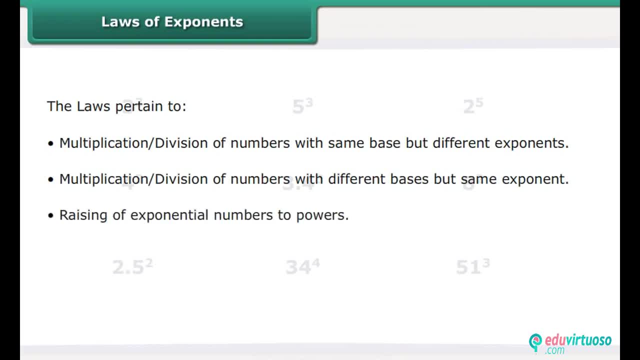 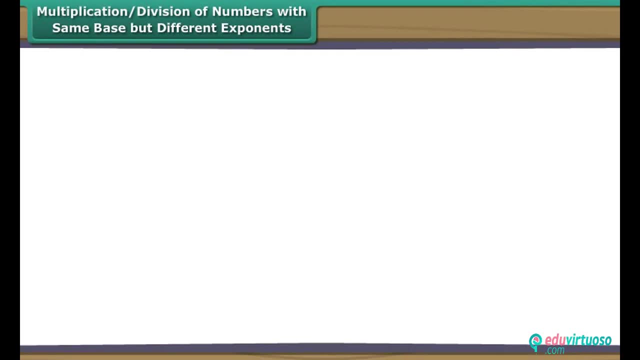 numbers in the same number. We can now see that the numbers in the same number are not the same, but their difference in dimension is not important. We can now find a common denominator of this exponential number. We can now can apply this equation: Multiplication, division of numbers with same base but different exponents. 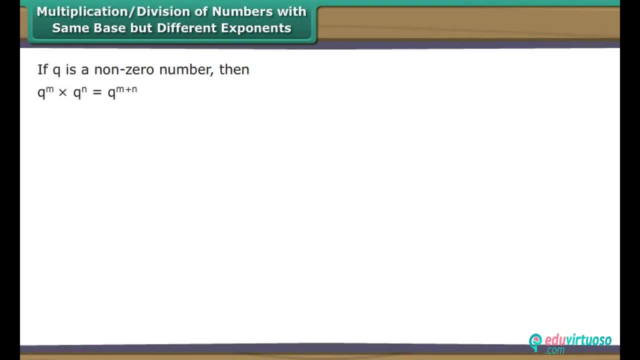 If q is a non-zero number, then q raised to the power m into q, raised to the power n is equal to q raised to the power m plus n. Product of two exponential numbers with the same base but different exponents, is an exponential number whose power is the sum of the powers of the multiplied numbers. 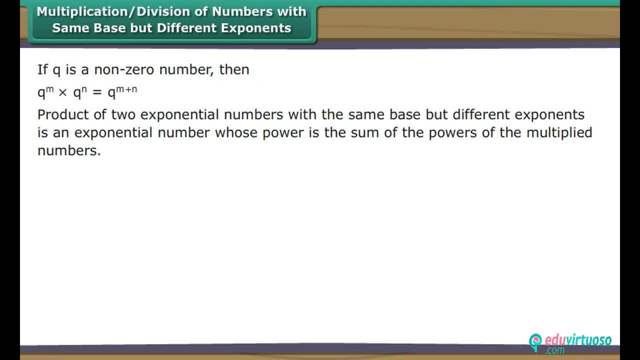 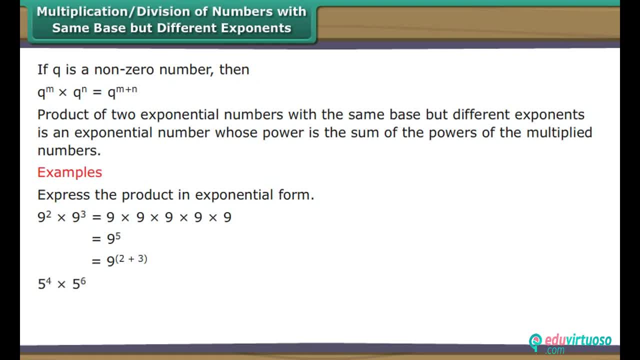 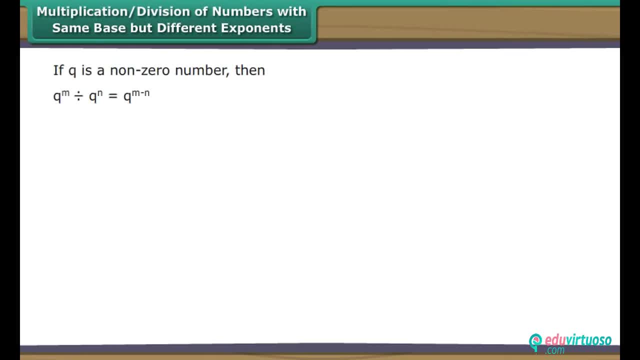 If q is a non-zero number, then q raised to the power m divided by q raised to the power n is equal to q raised to the power m minus n. Quotient of division operation between two exponential numbers with the same base but different exponents is an exponential number. 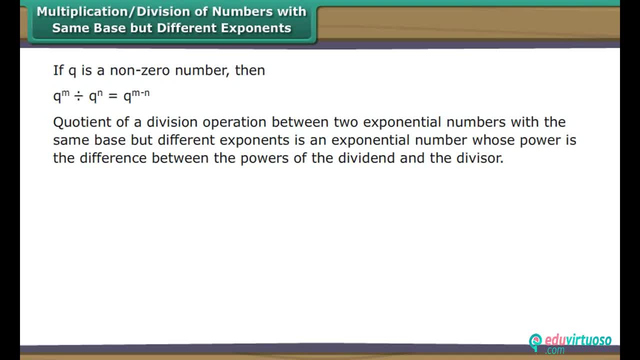 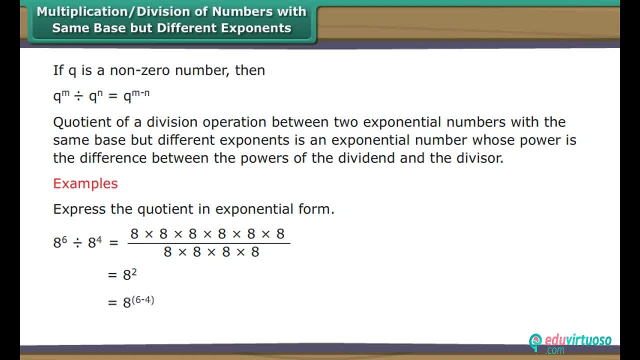 which equals 8 raised to the power 2 equals 8 raised to the power 6 minus 4.. 12 raised to the power 3 divided by 12 raised to the power 4 into 12, raised to the power 5, is equal to: 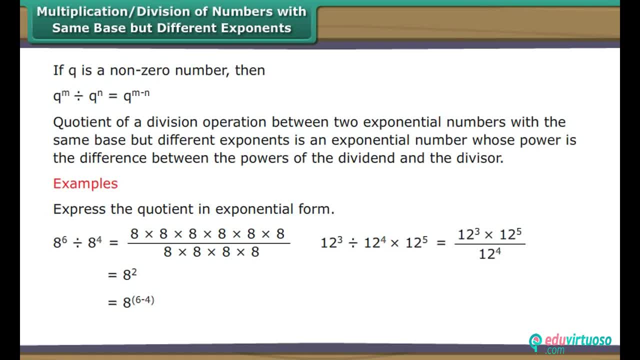 12 raised to the power 3 into 12 raised to the power 5 upon 12 raised to the power 4 equals 12 raised to the power 3 plus 5 upon 12. raised to the power 4 equals 12 raised to the power 3 plus 5 minus 4. 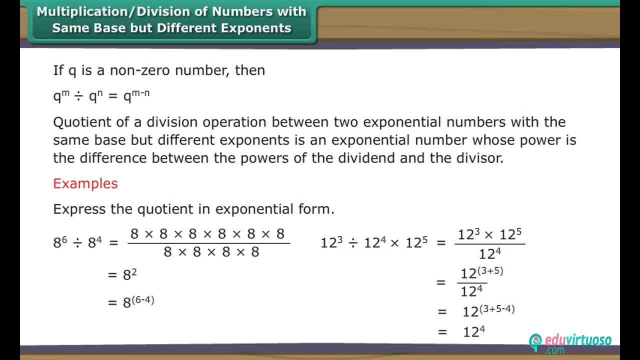 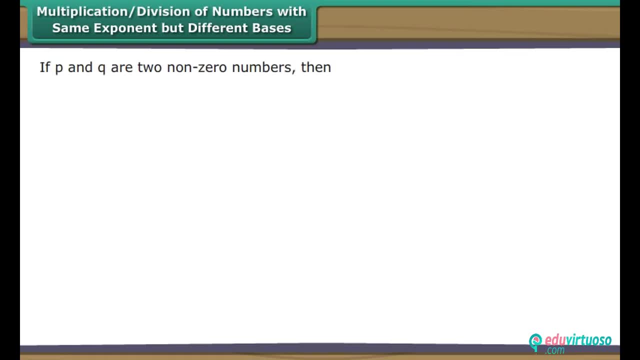 which equals 12 raised to the power 4.. Multiplication: division of numbers with same exponent but different basis. If p and q are two non-zero number, then p raised to the power m into q, raised to the power m, which is equal to p, into p into p. 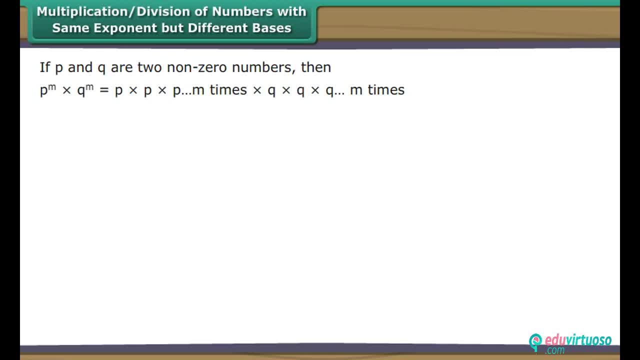 till m times into q into q into q till m times, which equals p, into q into p into q till m times, which is equal to pq raised to the power m, Product of two exponential numbers with the same exponent but different basis is an exponential number. 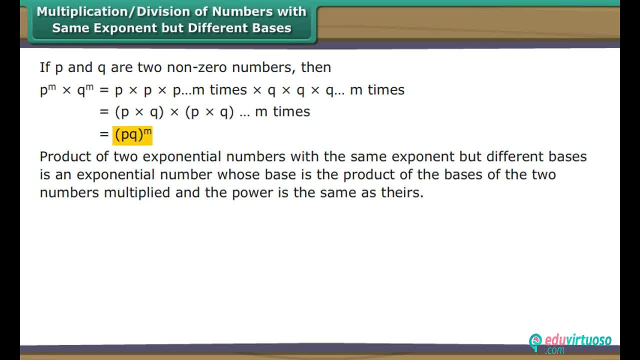 whose base is the product of the basis of the two numbers multiplied, and the power is the same as theirs. Let us understand this law with the help of some examples. Express the product in exponential form: 7 raised to the power 5 into 8 raised to the power 5. 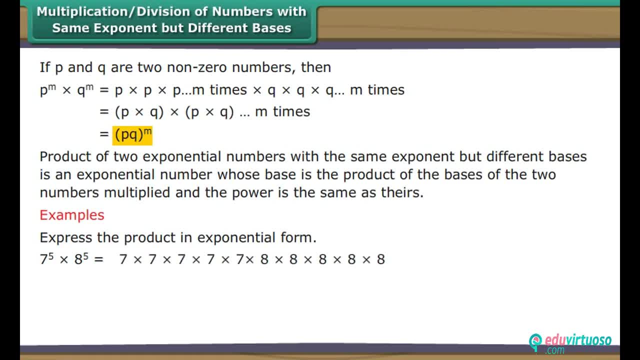 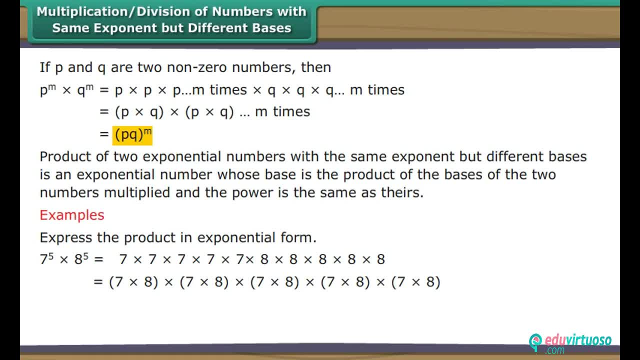 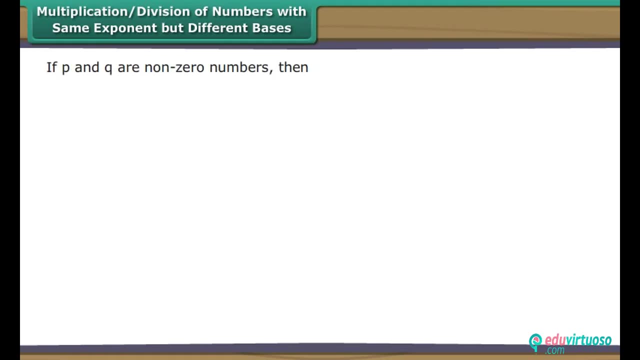 which is equal to 7, into 8 raised to the power 5, which equals 56 raised to the power 5.. If p and q are non-zero numbers, then p raised to the power m divided by q raised to the power m is equal to p upon q raised to the power m. 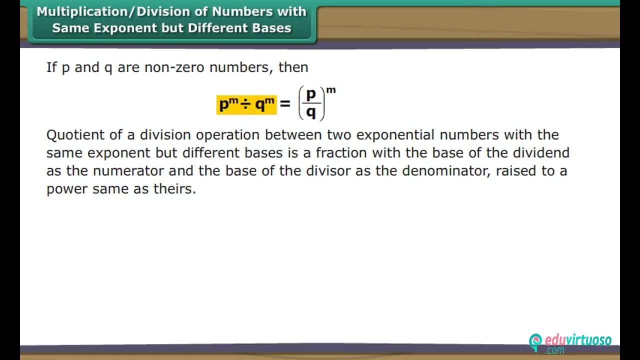 Quotient of a division is equal to division operation between two exponential numbers with the same exponent but different basis is a fraction, with the base of the dividend as the numerator and the base of the divisor as the denominator raised to a power same as theirs. 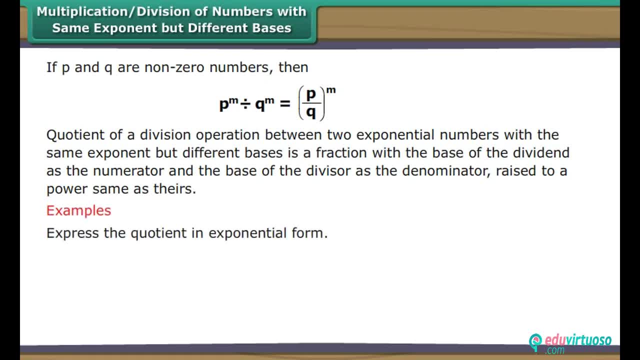 Let us now use the law. Express the quotient in exponential form: 9 raised to the power 6, divided by 4 raised to the power 6, is equal to 9 raised to the power 6 upon 4 raised to the power 6, which is 9 upon 4 whole raised to the power 6.. 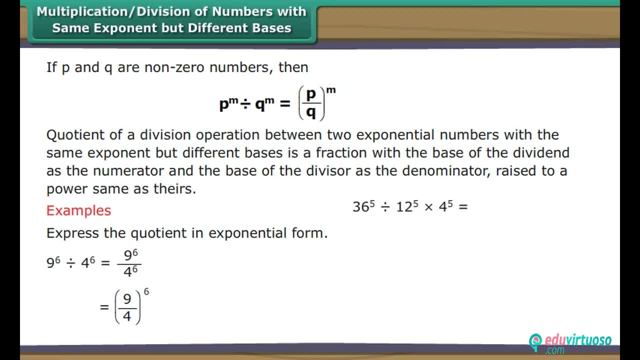 Similarly, 36 raised to the power 5 divided by 12 raised to the power 5 into 4, raised to the power 5, is equal to 36 raised to the power 5 upon 12. raised to the power 5 into 4 raised to the power 5, which is equal to 36 upon 12 whole raised to the power 5 into. 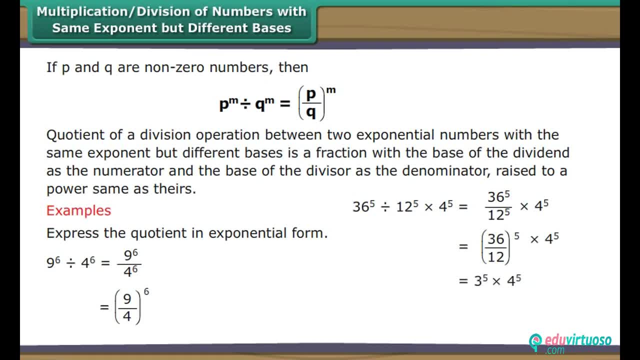 4 raised to the power 5, which equals 3 raised to the power 5 into 4 raised to the power 5, which is equal to 3, into 4 whole raised to the power 5, which will be 12 raised to. 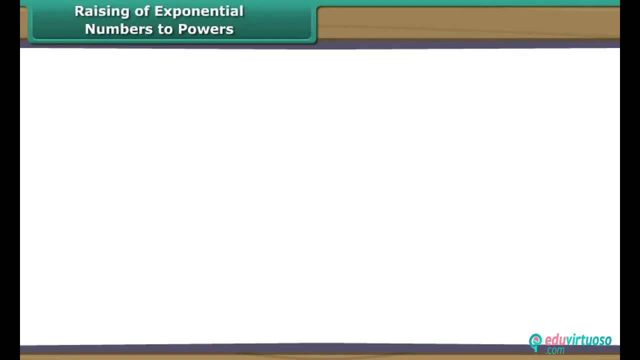 the power. 5. Raising of Exponential Numbers to Powers. If p is a number, then p raised to the power 5 is equal to power X whole. raised to the power Y is equal to P. raised to the power X into P. raised to the power X into P. raised to the power X into, so on till Y times. 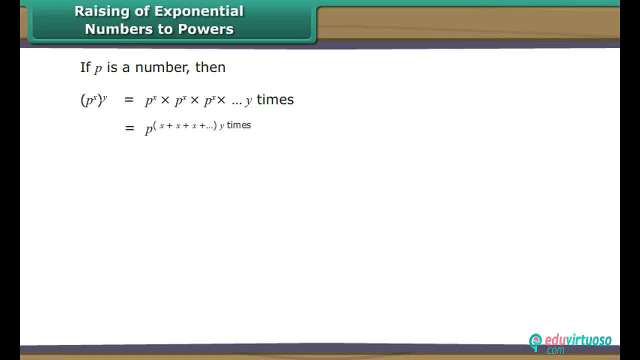 which is equal to P raised to the power X plus X plus X plus, so on till Y times, which equals P raised to the power XY. if an exponential number is raised to a power, the result is the base raised to the product of the two exponents as power. let us look at some. 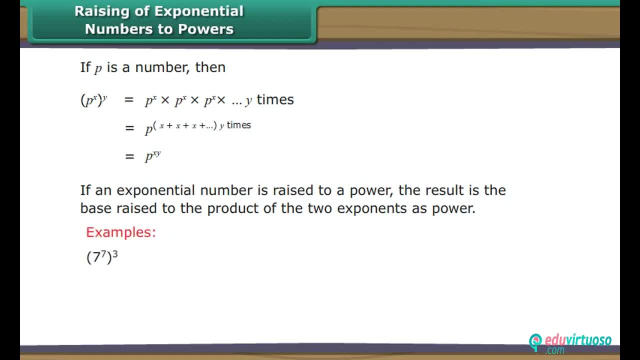 examples: 7 raised to the power 7 raised to the power 3 is equal to 7 raised to the power 7 into 7 raised to the power 7 into 7 raised to the power 7, which is 7 raised to the power 21, which equals: 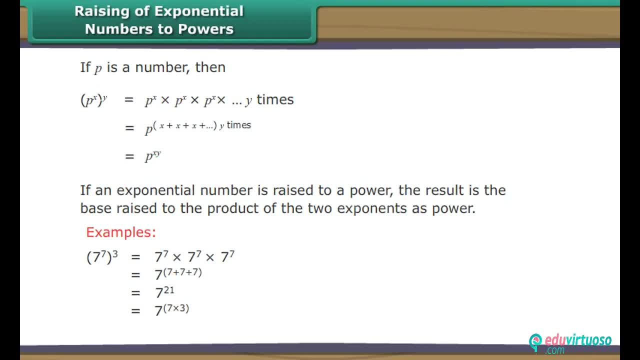 7 raised to the power 7 into 3. similarly, 24 raised to the power 3 raised to the power 5 is equal to 24, raised to the power 3 into 24. raised to the power 3 into 24 raised to the power. 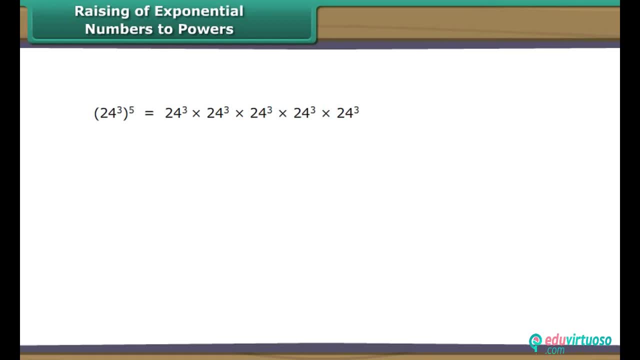 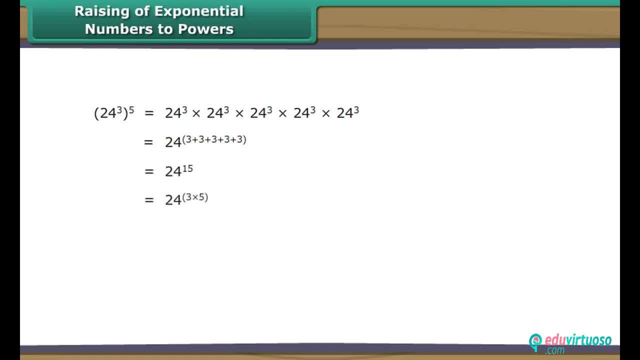 which is 24, raised to the power 15,, which is equal to 24, raised to the power 3, into 5.. Raising of a number to power 0. A number raised to the power 0 is 1.. If S is a number, then S raised to the power 0 is equal to 1.. 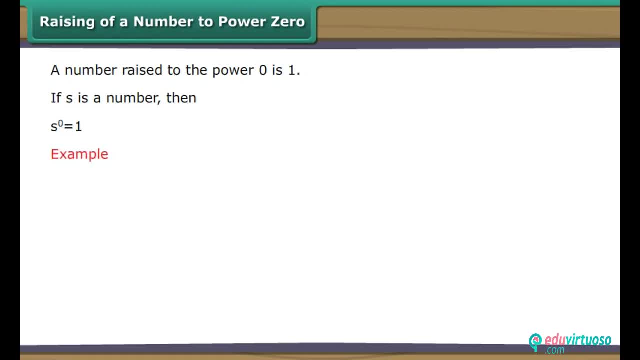 Let us solve some questions based on exponent 0.. Simplify What is common among these numbers: 9.8 into 10, raised to the power 3.. 7.3 into 10 raised to the power 4.. 5.82 into 10 raised to the power 5.. 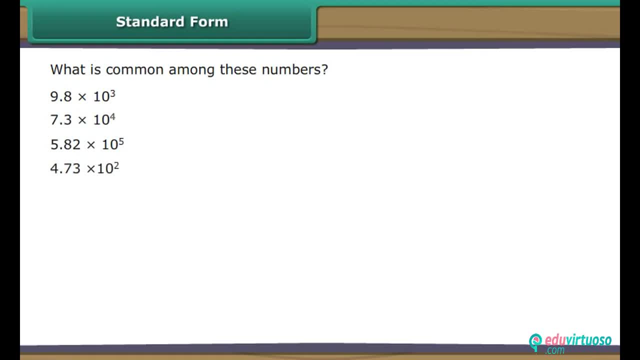 4.73 into 10 raised to the power 2.. All of them contain decimal numbers between 1 and 10 multiplied by powers of 10. Numbers that are expressed as products of decimal numbers between 1 and 10.. 1 and 10 and powers of 10 are said to be in standard form. 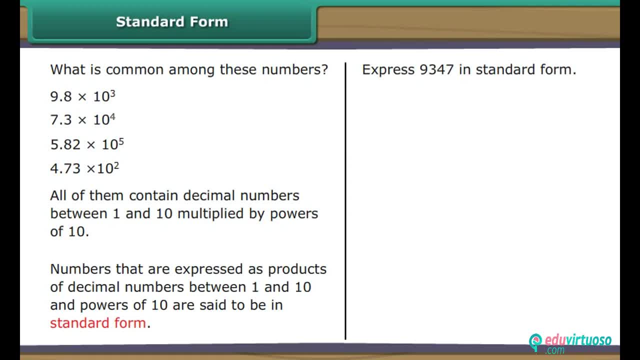 Express 9,347 in standard form. 9,347 is equal to 9,347 upon 10 cubed into 10 cubed, which is equal to 9,347 upon 1,000. into 10 cubed, which equals 9.347.. 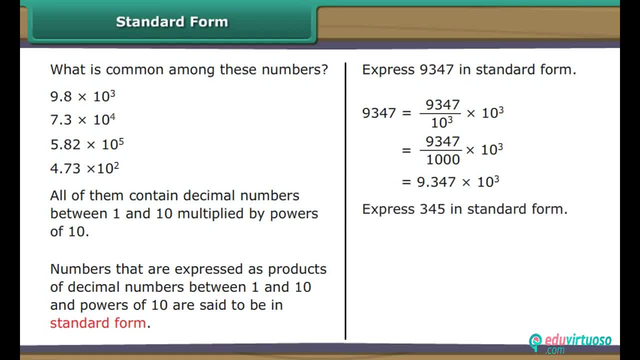 Now express 345 in standard form. By simplifying it, we get 345 upon 10 squared into 10 squared, which is equal to 345 upon 100 into 10 squared, which equals 3.45 into 10 squared. 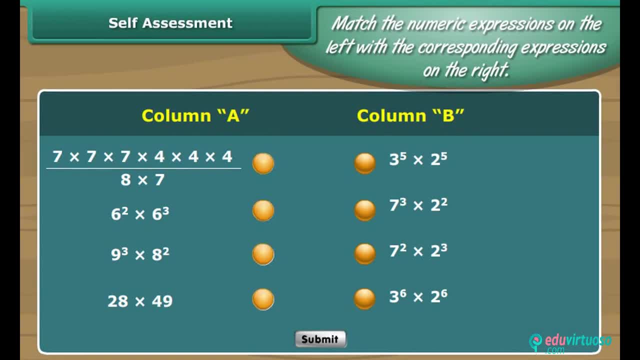 Self-assessment. Match the numeric expressions on the left with the exponential forms on the right. Again, we express the number totally perch note- as if we were expecting a pase. in order to effectively understand the operation procedure, We need to hit known values- 4, and then the exact situation, function and average. 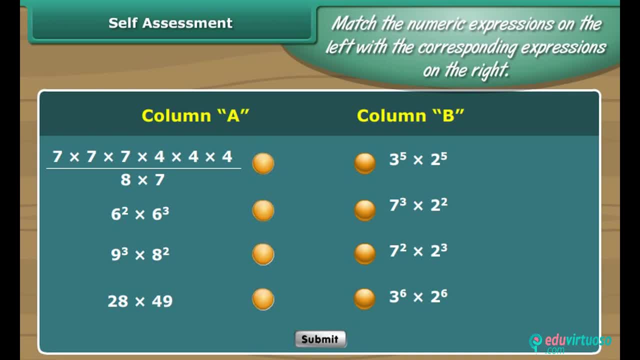 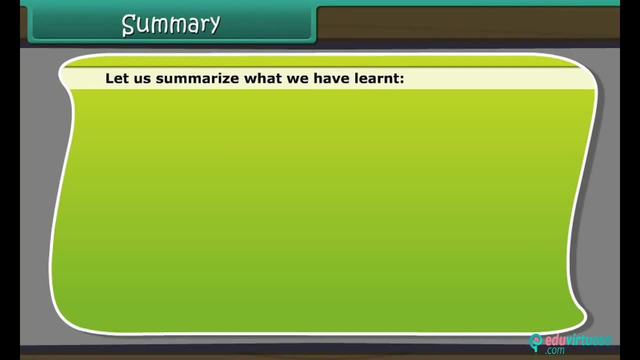 cost per second. to come back to the basis calculated by atoms, which is assumed to be slightly higher than the average Summary, Let us summarize what we have learned: 3. 1. 3.. 1 per second: 2.. 1,3,5,5,6,6,7,5,6.. 3. 2,3,5,7,6,5,6.. ienzaat imitabars h. 2. 1 pi h.